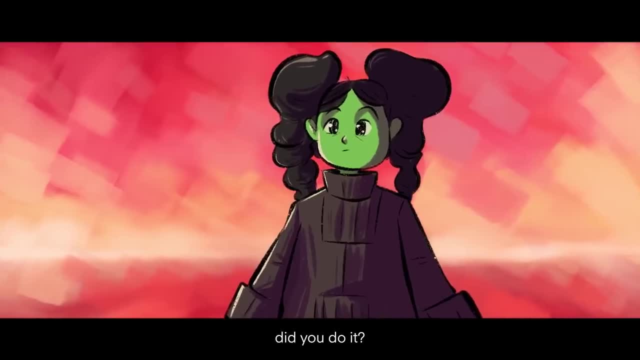 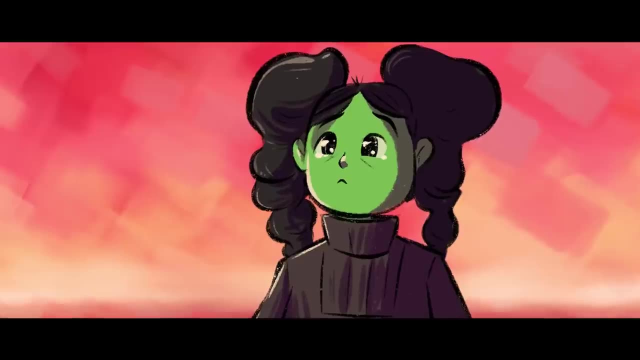 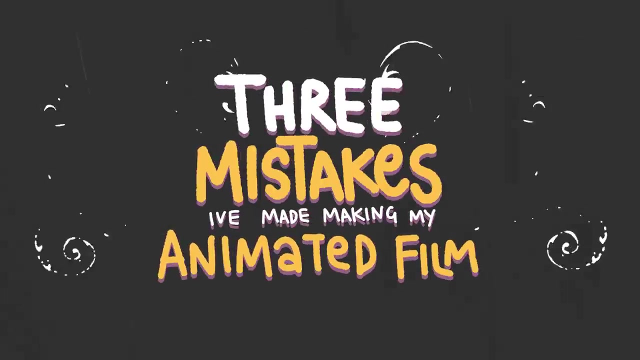 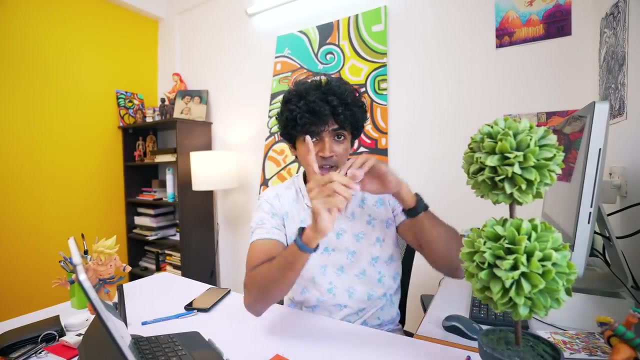 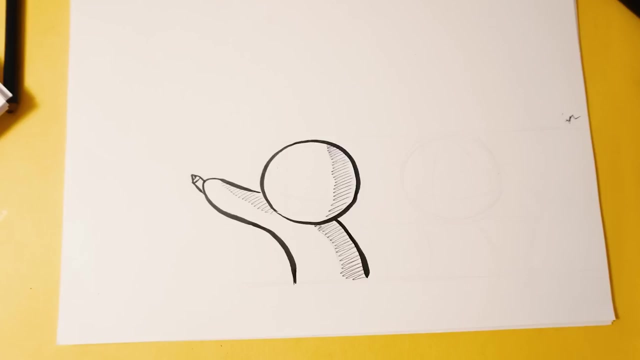 So here's the first mistake that I have made, thinking that I need to make my first short film really good. So I was wanting to make an animated short film for three freaking years and I didn't do it. Why? Because I thought the first short film that I've ever made should be really crafted, really. 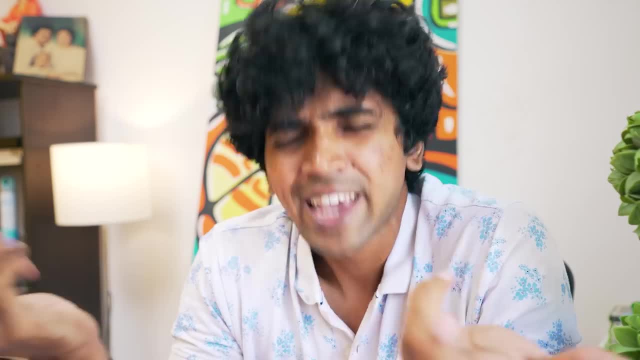 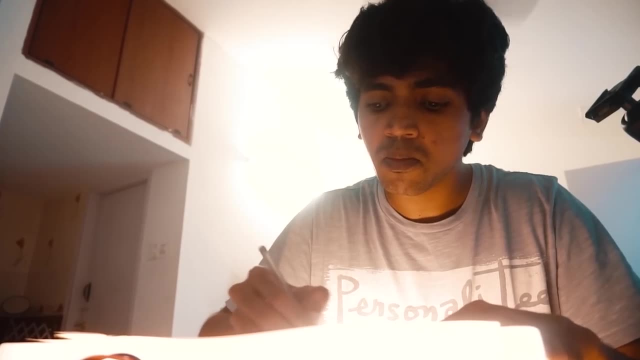 well-defined, really perfect. It should be really, really, really good. It can't be. actually It can be, and I've tried, and it wasn't Why? Because I simply did not have a skill, because I did not put enough repetitions to get good. 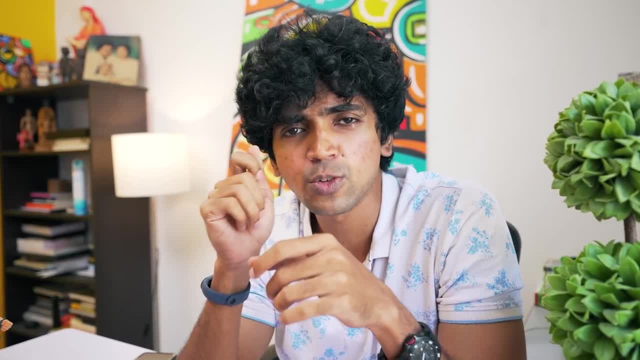 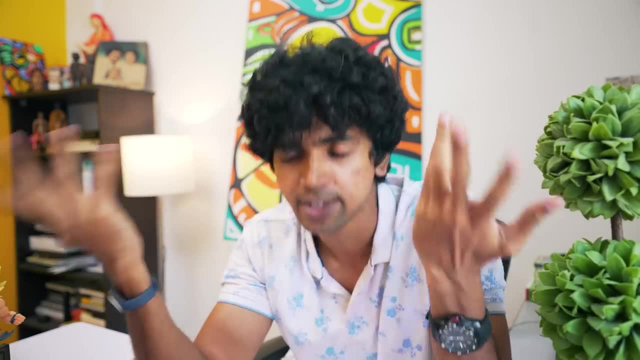 If I need to have put that repetitions in, I should have started with my first short film, which I did not do. How can I get good at something if I did not start doing it? Here's what I should have done instead a long, long, long time ago. 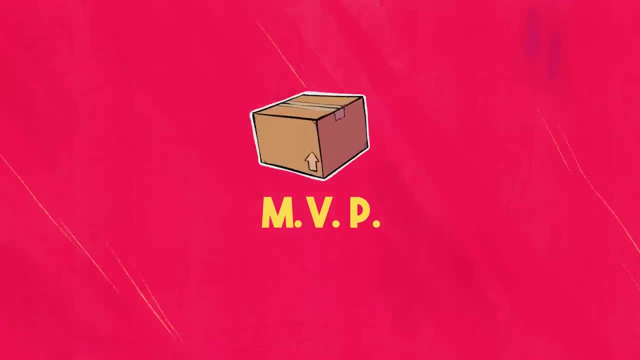 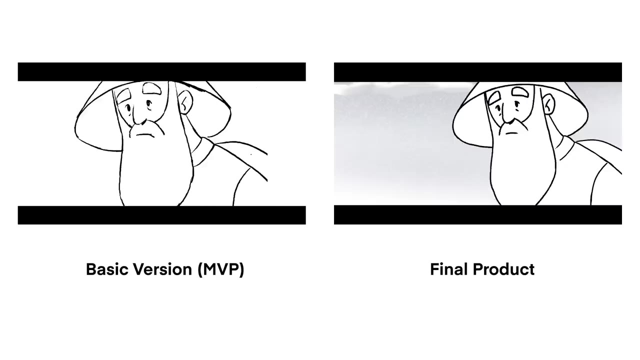 I should have gone ahead and created an MVP. What does that mean? It means a minimum viable product. It's a term often used in the business and startup cultures. It's a product that is simply the most basic version of your larger product that just captures. 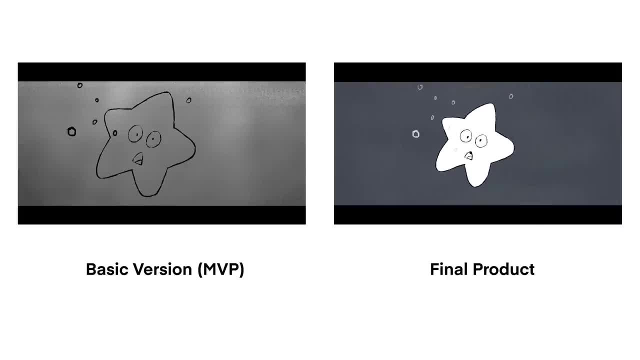 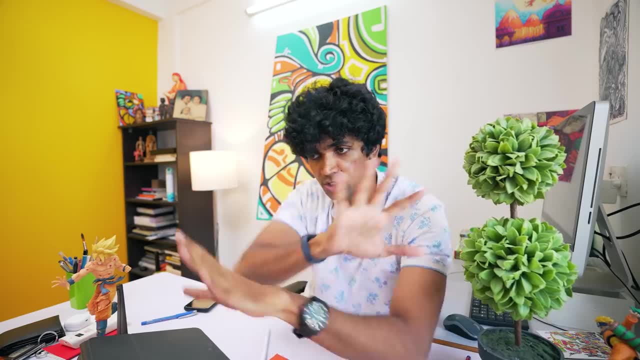 the core essence and the necessities in the most minimal fashion Just works. That's an MVP. So that's why I did. I just stopped what I was doing Generally, all the projects that I was doing as I put a stop. let's stop it here, guys. 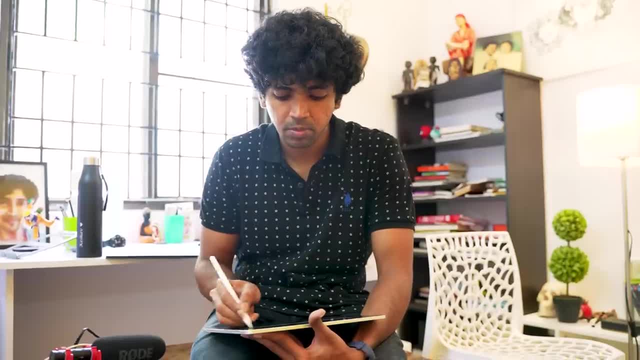 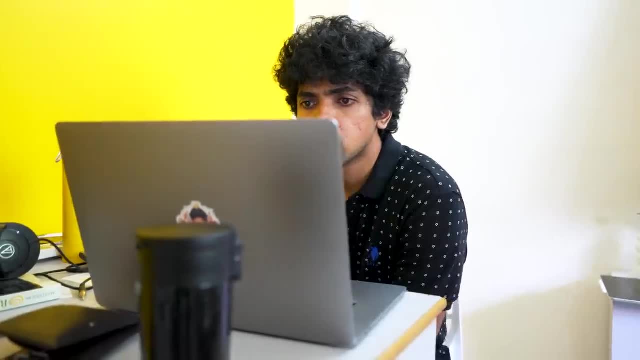 Let's just focus on making a short film in 48 hours. Let's make the shittiest, crappiest version of the short film that we possibly can. that just shows what this thing can do in 48 hours, And then, heck, we'll refine it in two weeks. 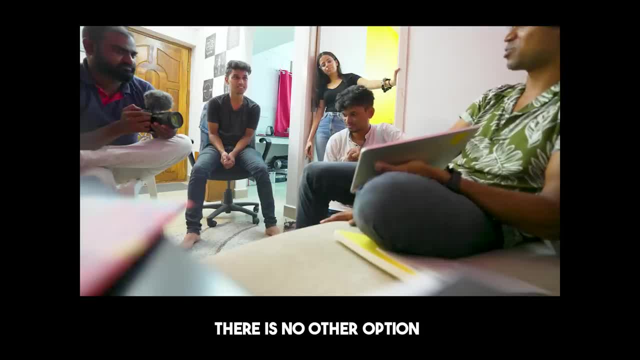 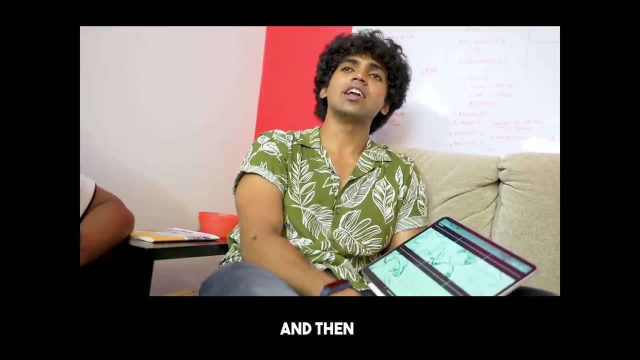 We have to finish this, which I want to finish it. There's no other option. We have to finish it. That means let's just make it black and white. Let's finish this and then fill in all the colors And then make it color. 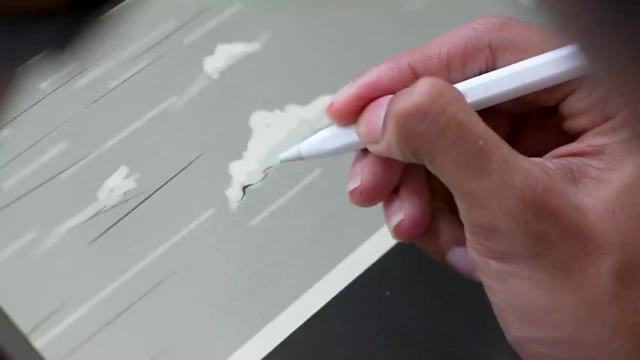 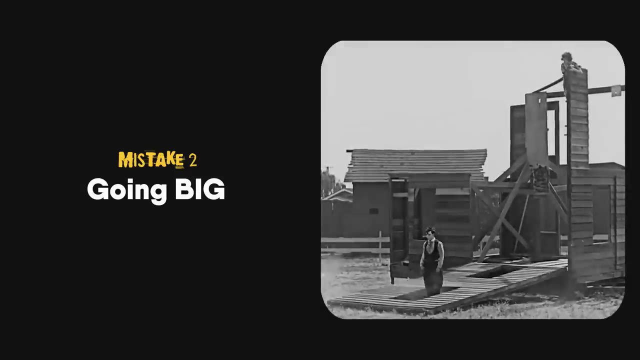 Still, it's a very short period of time to put my first quality or decent work out there. Second mistake is this: Don't take on something that is too big at the start. So I made this mistake a couple of times in the past. 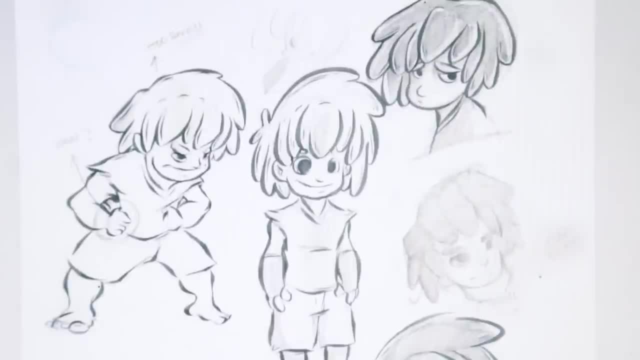 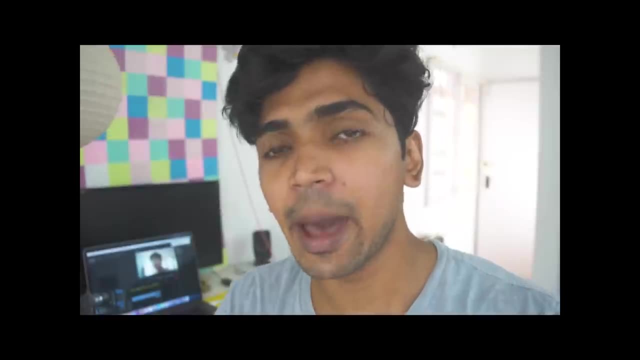 In 2018, I took on this comic project, My Avatar. That's basically it. It's my big life project And I took that comic project as my first ever project. And guess what happened? I am putting my 100 days of making comics. 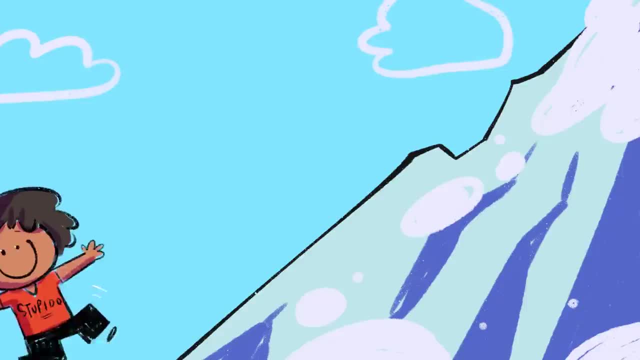 I am putting my 100 days of making comics. I am putting my 100 days of making comics on home. It's too hard. It's too hard to climb Mount Everest on day one If you haven't ever climbed or been on a hike before. 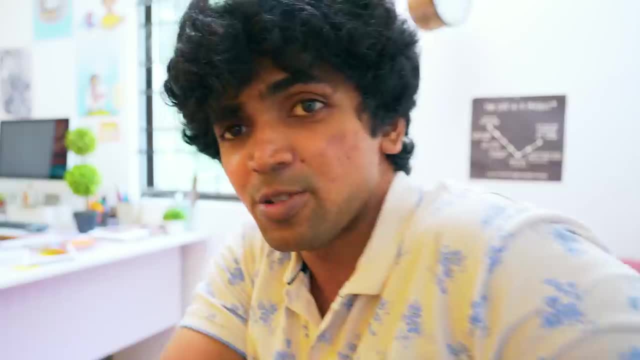 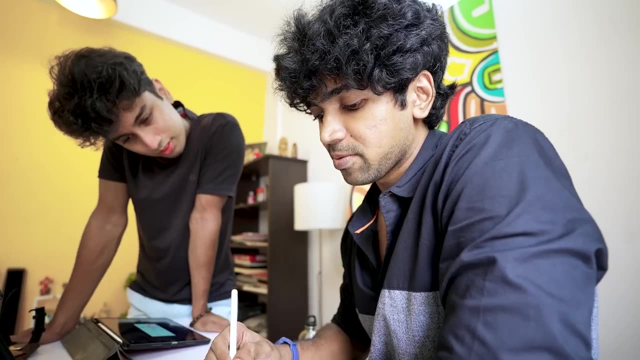 Right, Because I was that kid- I had never been on a hike before Then. I was taking on a big project- Was sort of going to do that same mistake right here as well, But I was more aware of my mistakes this time. 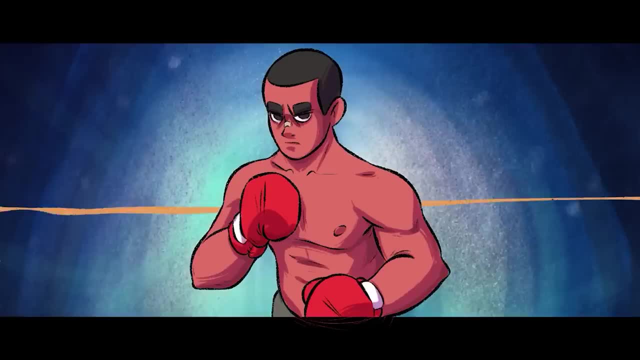 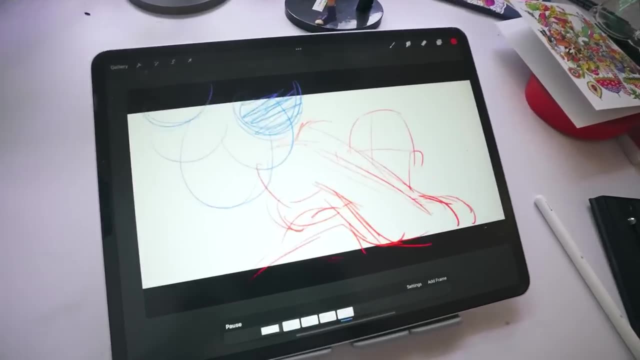 I took on a one minute short film, a one minute very small color short film called Sweat and Blood, And I thought: you know what? It's not my Mount Everest, It's very simple, It's just a hike. i was wrong, so we've been making a super short short film right, which is one minute long apparently. 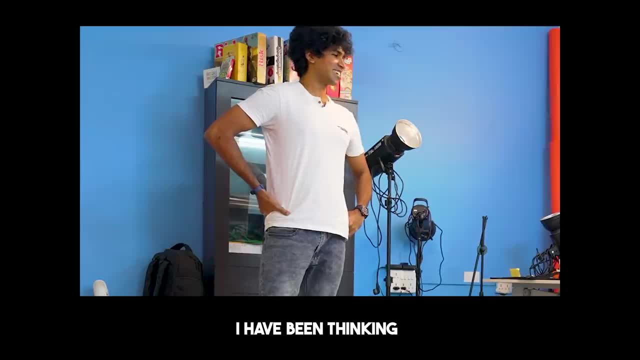 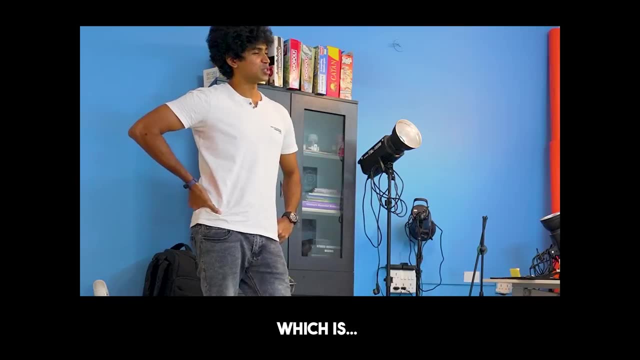 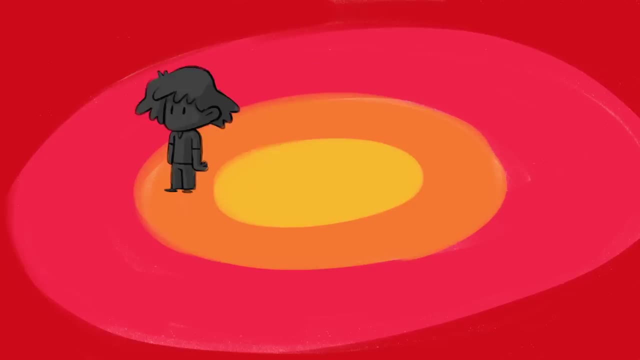 it's taking a lot of time, as you can see. so i've been thinking, which is not a good thing, i don't know. i've been thinking what doing it, which is make something even smaller, make something even more doable- what is my comfort zone and what is slightly outside of my comfort zone, and pick. 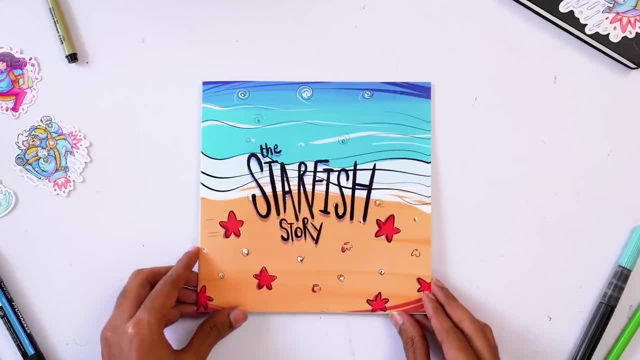 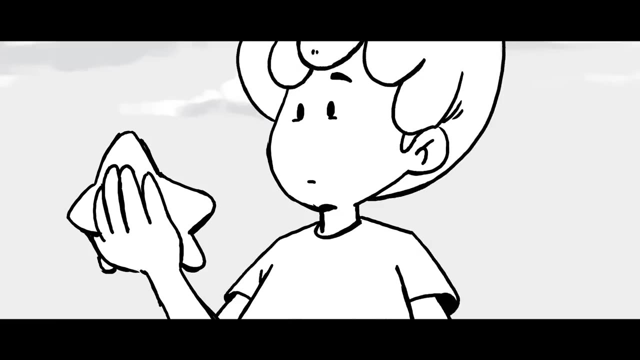 that thing. so for me, it was this five hour comic that i made in the past. it was a very short comic with a very simple story, and i was like you know what, let's make a very small, very doable short film. and this time let me make it even easier on myself by hiring other people, hiring an animator. 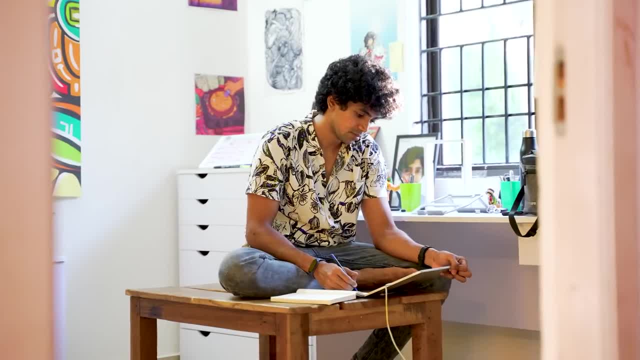 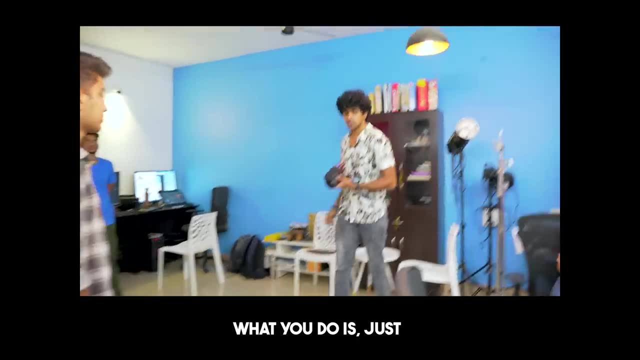 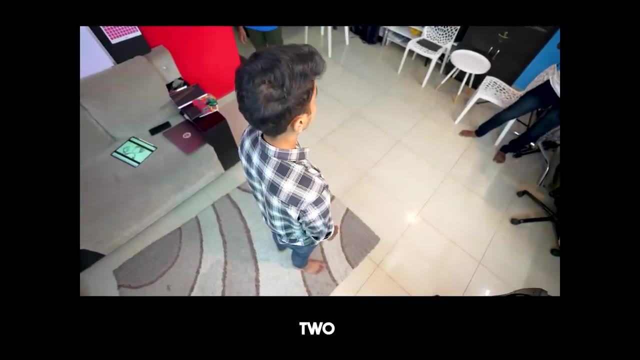 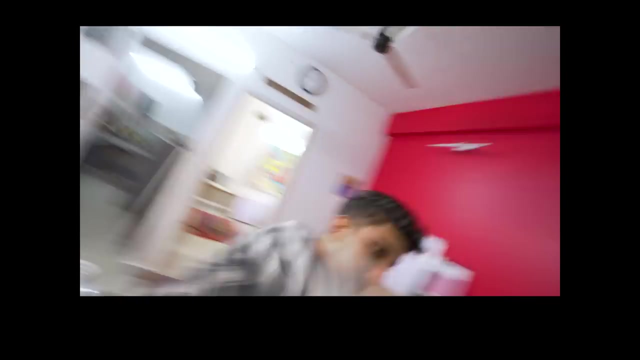 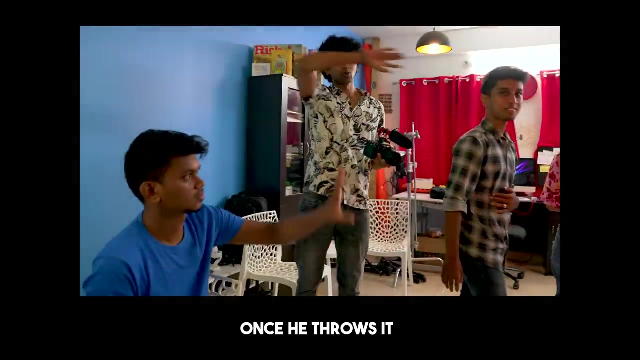 getting an animator who's got some experience so that i can actually focus on character design, directing keyframes and all those things. what do you do is just just two and then flip it like this: ready three, two, one go. ready, three, two, one go. once he throws it, the guy is like looking: go like that, and then the starfish. 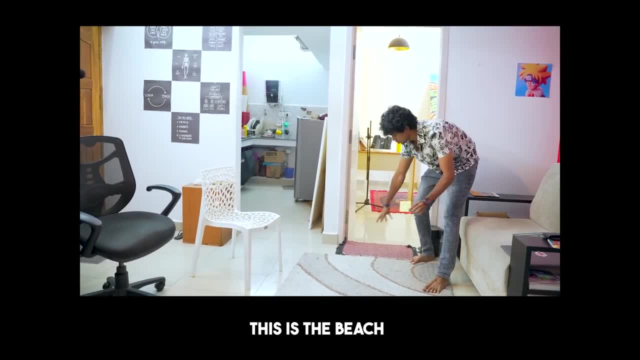 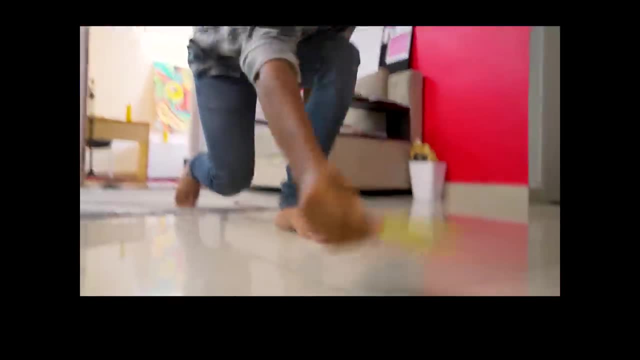 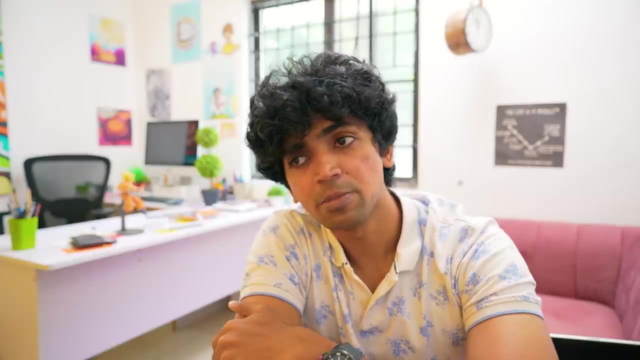 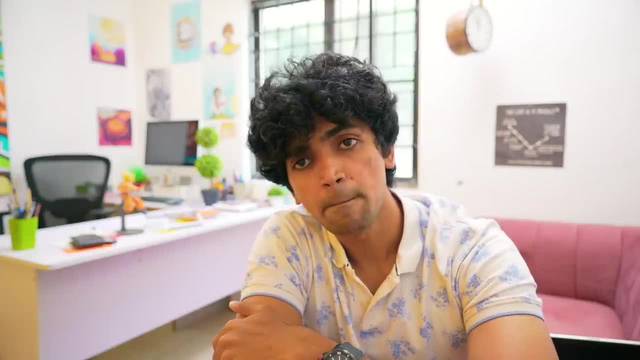 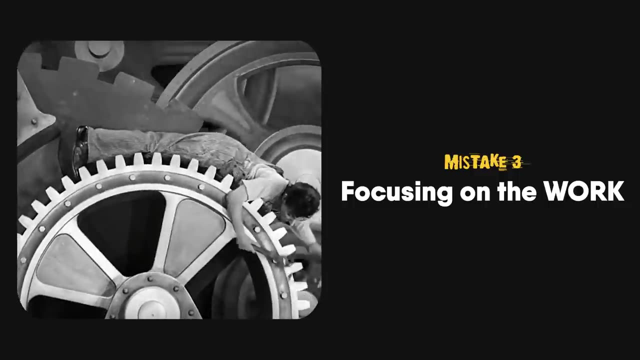 taking something more doable, slightly outside the comfort zone, is much better because, my friend, there's a more important thing than the work that you make, which is the kind of person that you become. that is the third lesson. by the way, if you bring a millionaire to the streets, they will still 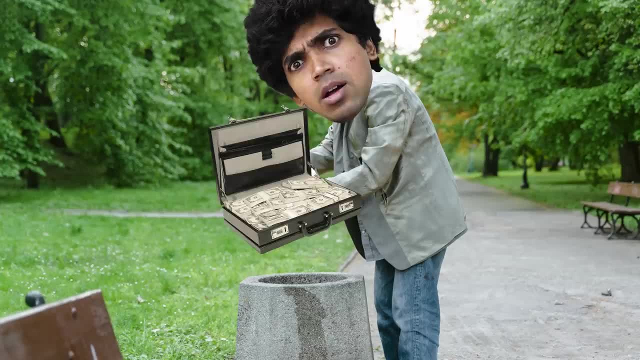 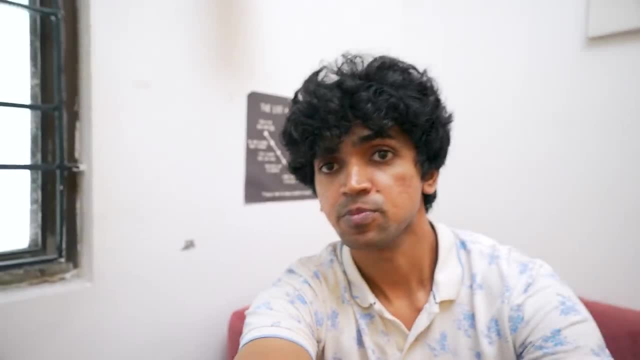 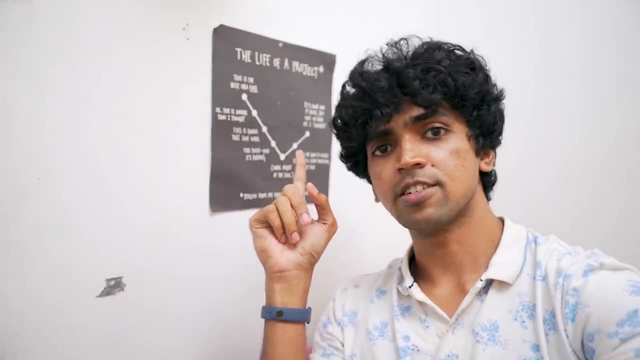 become a millionaire after a while, but if you give a poor person a million dollars, they would still become poor. let me show you something. see this. this is what i call the project cycle. it's from austin cleon and it actually shows what the life cycle of a project sort of looks like if a person tries really, really hard and 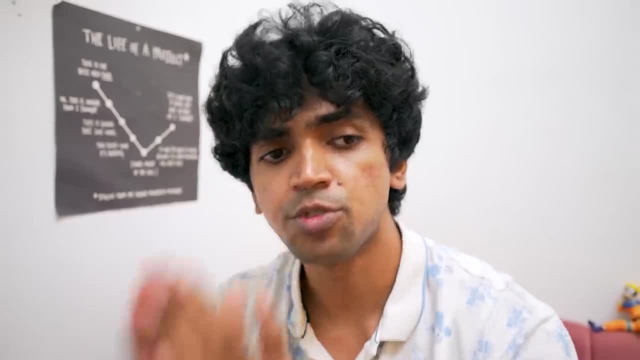 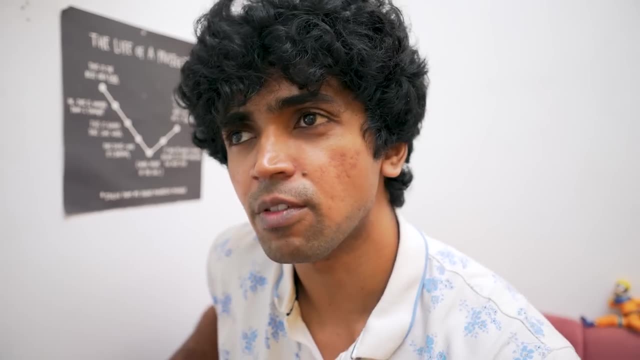 they put in all the effort and make this one great piece of work, one great piece of short, one great piece of artwork. they just go through that project cycle just once, whereas if you do more work and focus more on the art and the design, then you're going to get a lot of work. 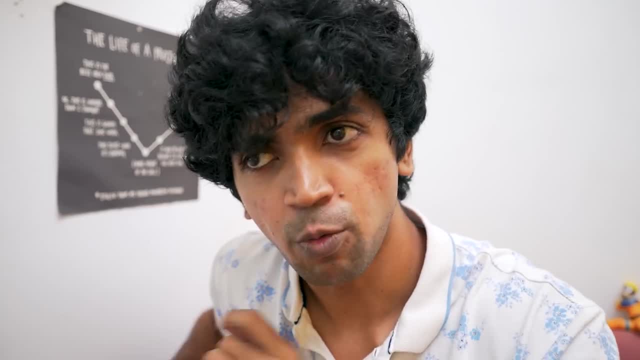 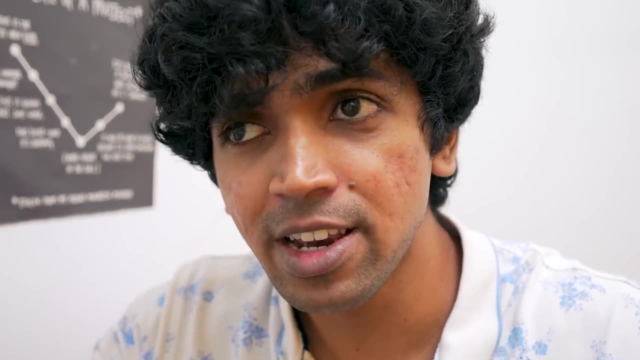 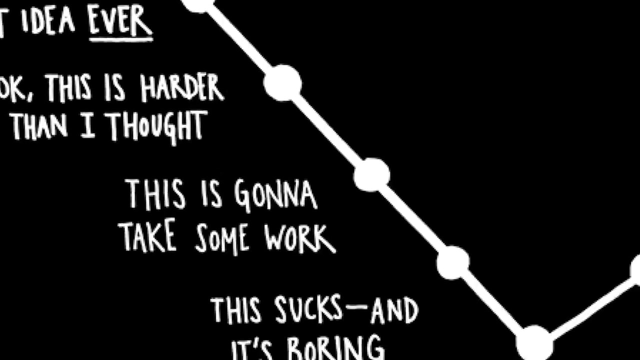 and then you're going to get the whole thing done. okay, do more repetitions of work, more volume of work, probably less shorter in quality, so that you can actually get more volume right, get more repetitions in. if you do that, you will go through the project cycle of actually finishing something multiple times, because in life cycle, the life cycle of 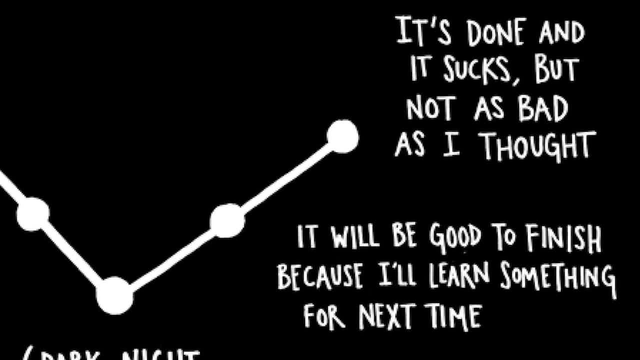 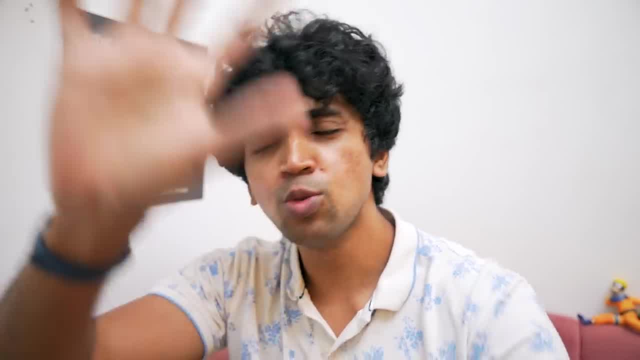 the project, to my understanding and to my knowledge, involves so many emotions, so many ups, so many downs, so many struggles that will just make you go off track very, very, very easily. but you realize that you are essentially your own biggest enemy in a given project for you to stop. 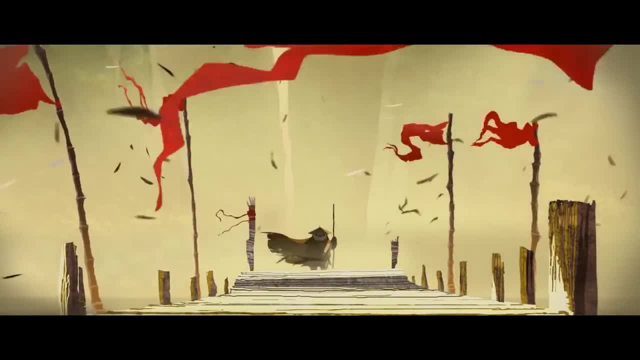 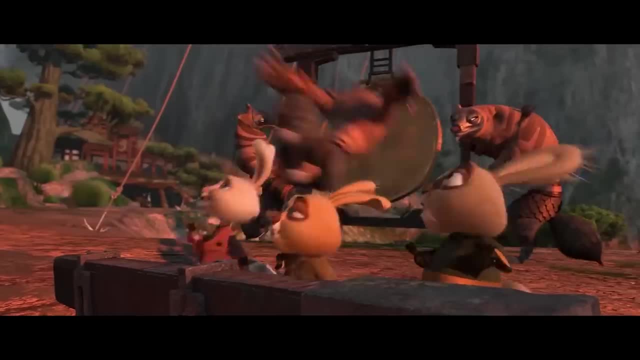 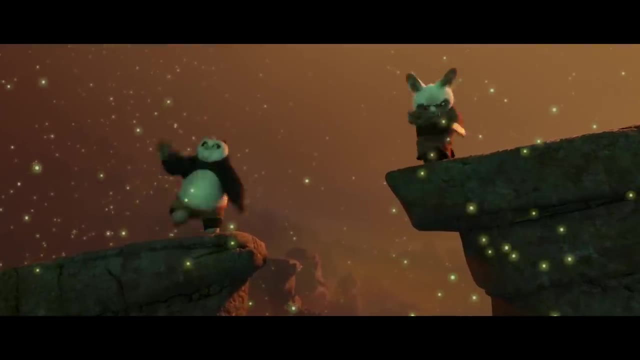 being your own biggest enemy. you have to actually become a seasoned warrior- seasoned warrior with battle scars, who's gone to war so many times that they can actually- you know- see through all the bull crap that you throw at yourself and stay focused on the task at hand and actually have